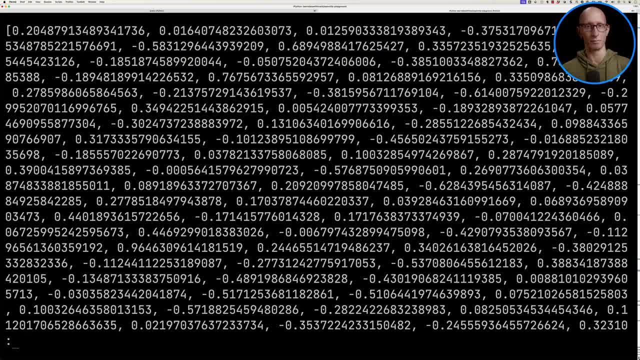 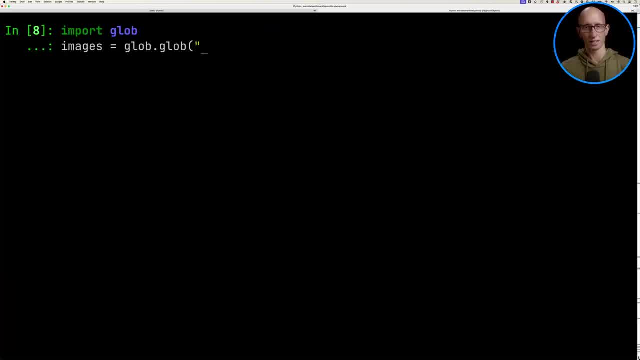 going to embed that image and you can see it comes back with a bunch of numbers as well. now let's have a look if we do this for some more images. so i'm going to just load all the images in my images folder that have the png extension into an images file and if you have a look, you can see i've got a lot. 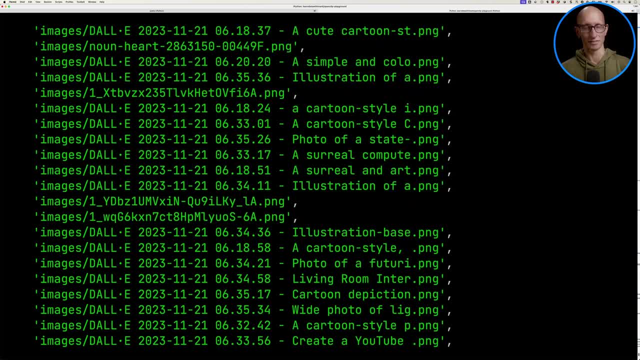 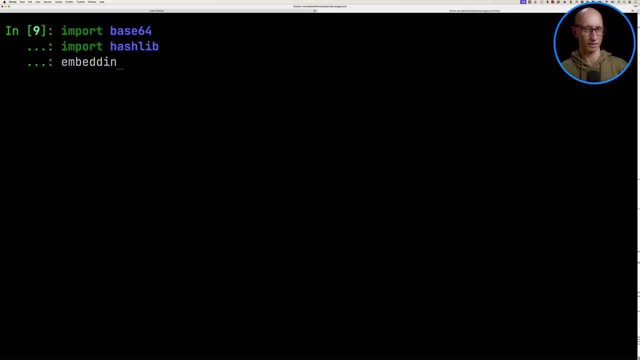 i've been using dali a lot. i've got a lot of images coming from there and what we're going to do now is embed all of those. so we're going to just import the base64 and hashlib functions. we'll create an embeddings array and then we're going to iterate over our images, open each one. 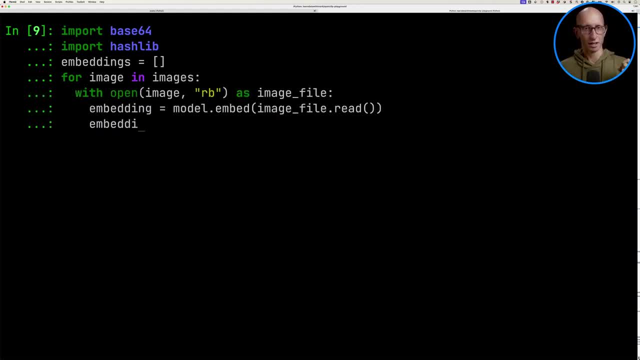 create an embedding and then we're going to put it into the embeddings array and we're going to have a dictionary. so we'll have an embedding, we'll put a path and then we're just going to generate an idea, like a same size ID, based on the image path. we're going to put these. 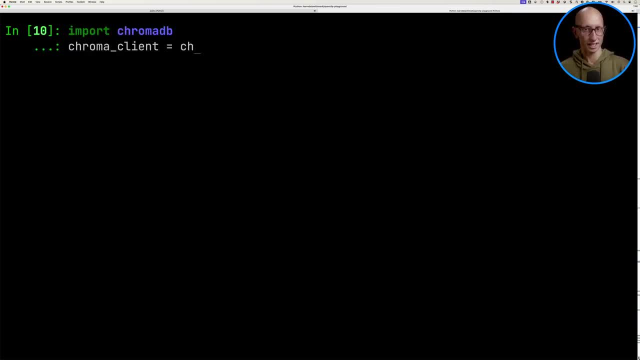 images into chromidb. so we're going to import chroma, we'll create a client, and then we're going to create a collection called images, and then we're going to add the images to the collections. so we'll start with the embeddings, then we're going to create the metadata, which in this case is going to be the file path, and then 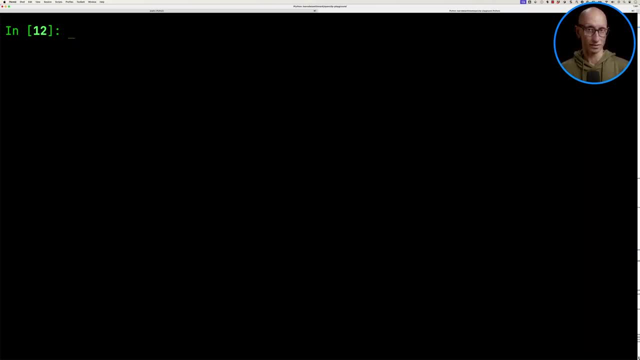 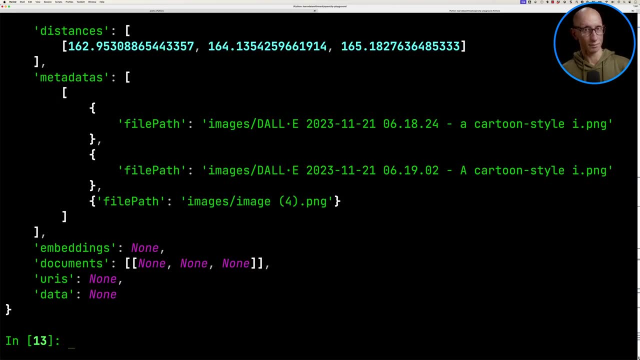 we'll give them the ids as well. now let's do a query. so we're going to again, we're going to create an embedding for the cute dog. then we're going to query the collection and get three results and you can see it comes back with the results. we've got the distances and then underneath we've got the the. 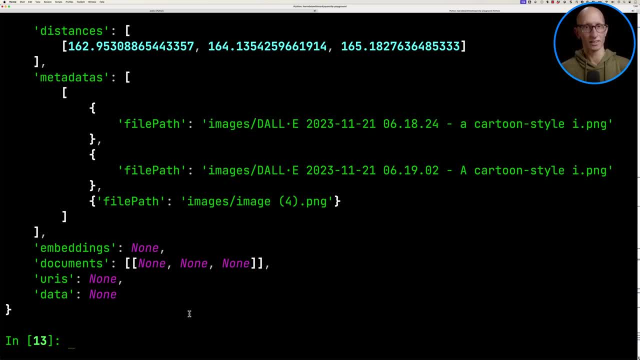 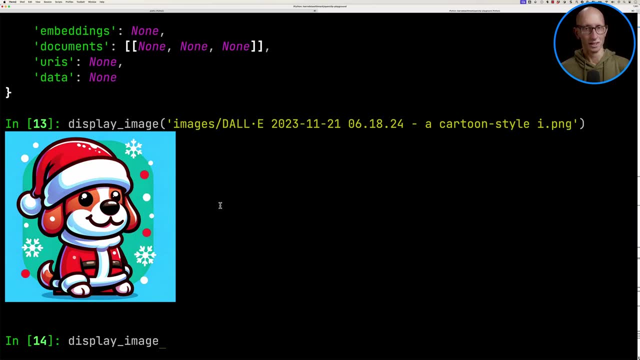 metadata, and if we copy the file path for the first result, say, and then use our display image function, you can see that it comes back with with the dog. how about if we do it for the second one as well? so this time it comes back. it's probably quite cute. but it's not a dog, right, it's an owl. 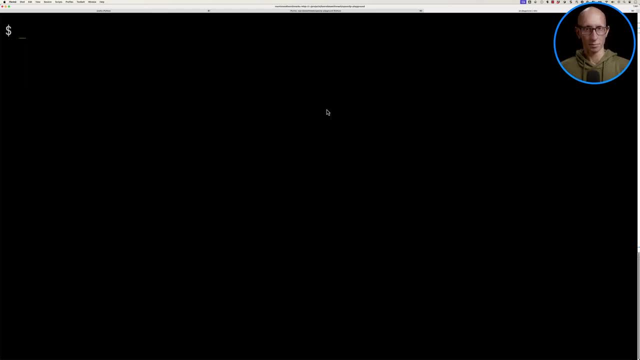 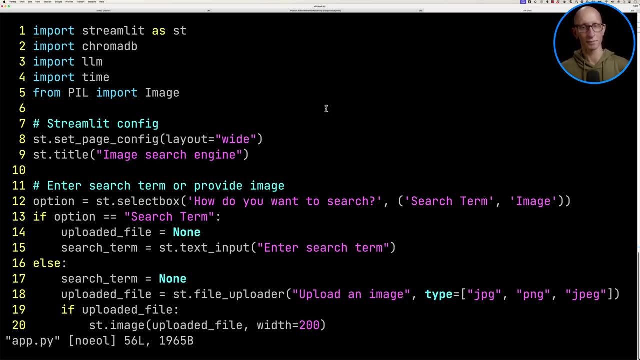 and a walrus. let's now have a look at how we would put this into an app. so we're going to open a an app, the apppy file, where we've got a streamlet app, and i'm not going to code this from scratch, but i'll just show you something that we built earlier. so at the top we've got some imports. 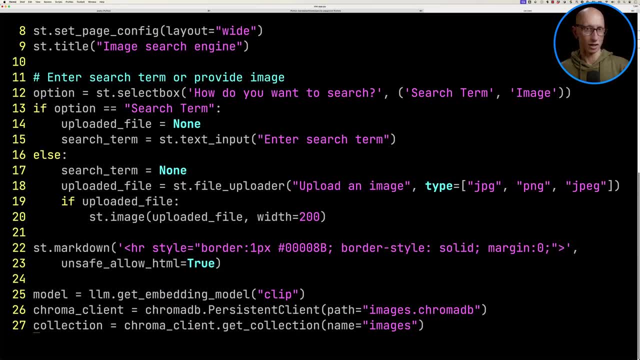 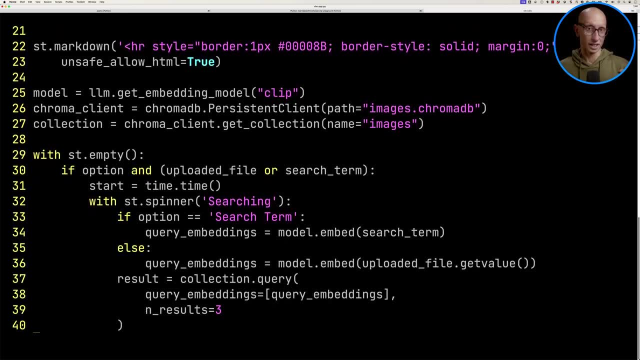 we've then got our streamlet config. if we come down a little bit we can see we've got an ability to choose a search term or upload an image, and then we've got just a little divider and then we load in our embedding model the clip embedding model and the chroma client.